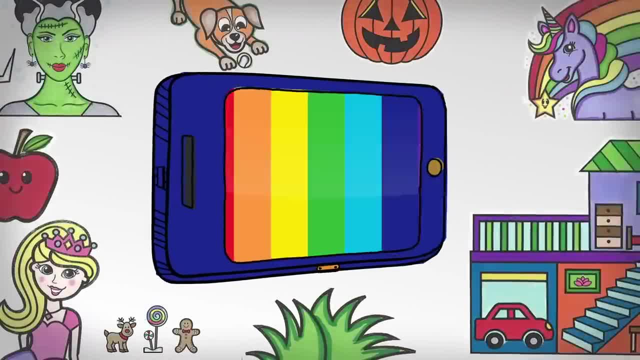 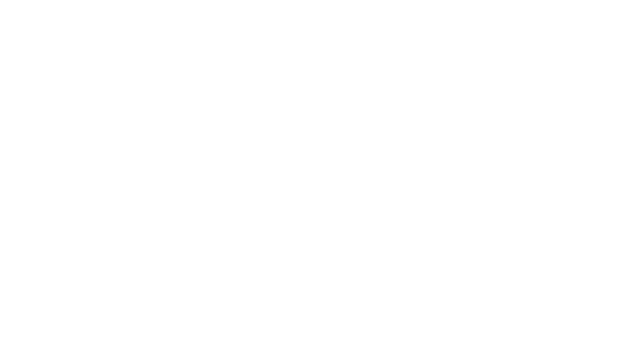 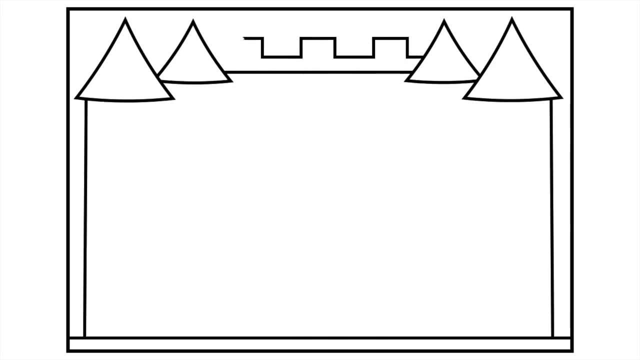 Hi everybody, Welcome to Colorful Creative Kids. Would you like to have some fun and color with us? If so, you're in the right place. Let's get started. Hi everybody, Welcome to Colorful Creative Kids. Would you like to have some fun and? 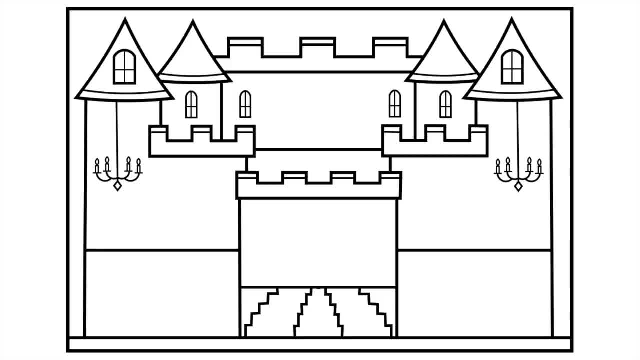 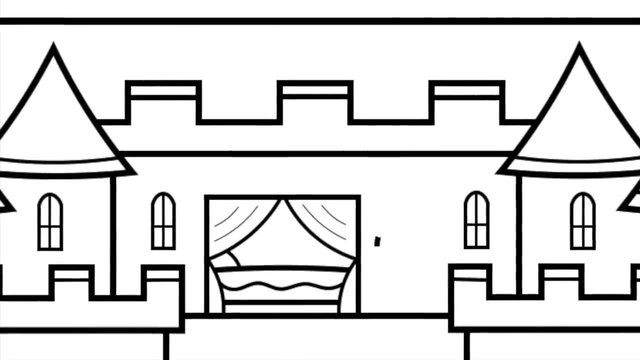 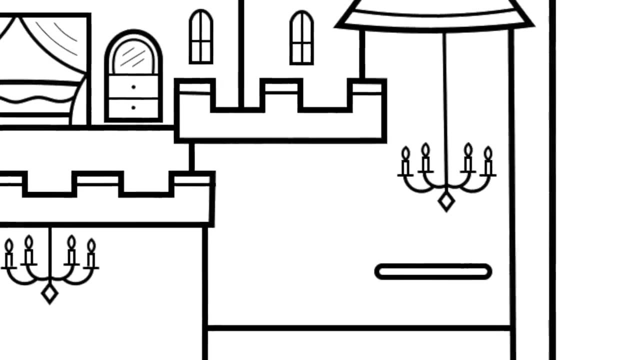 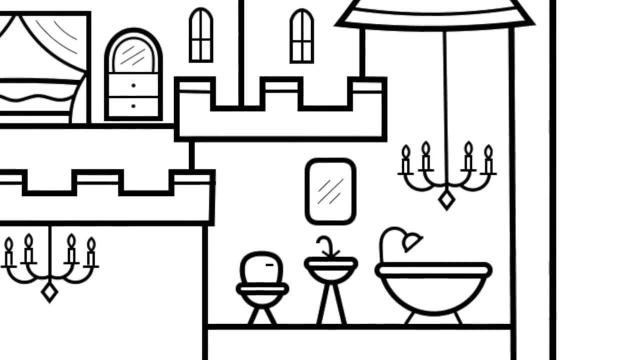 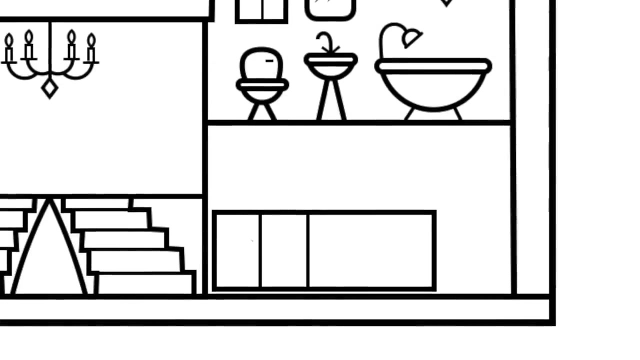 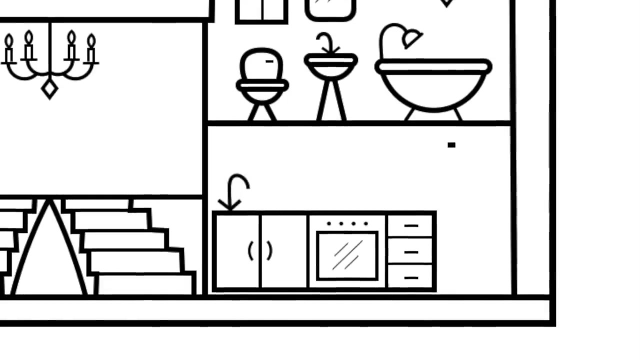 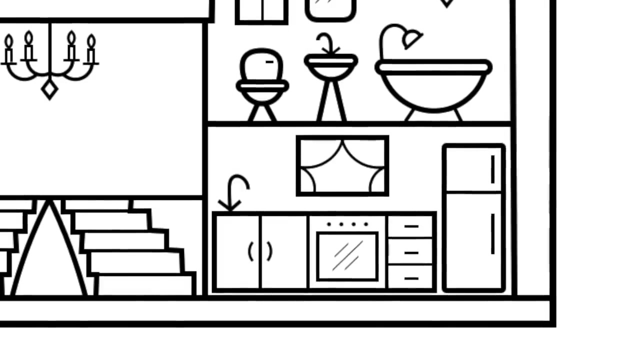 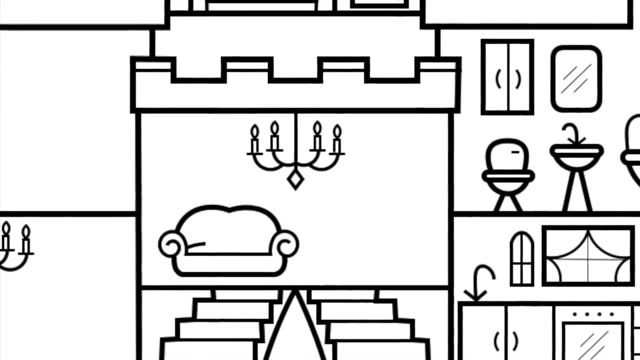 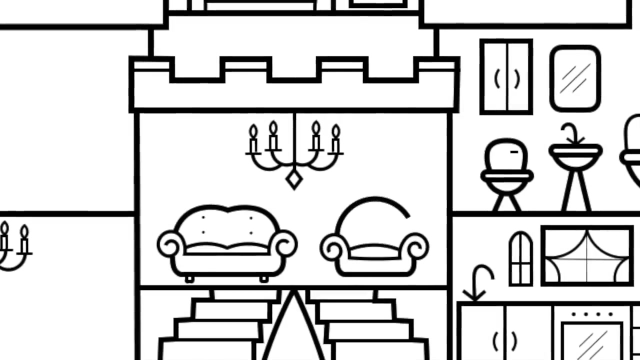 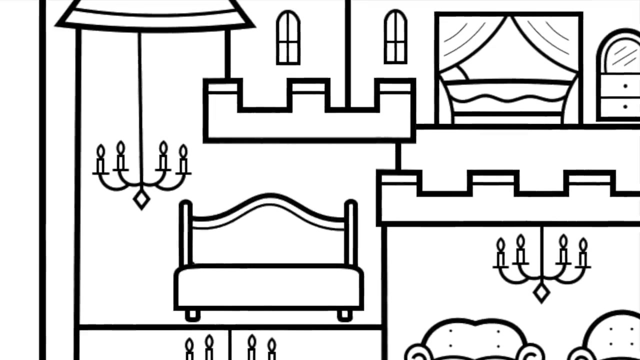 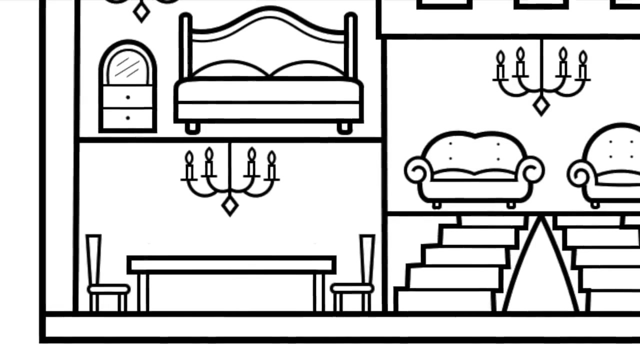 color with us. If so, you're in the right place, Let's get started. Hi everybody, Welcome to Colorful Creative Kids. Would you like to have some fun and color with us? If so, you're in the right place. Let's get started. 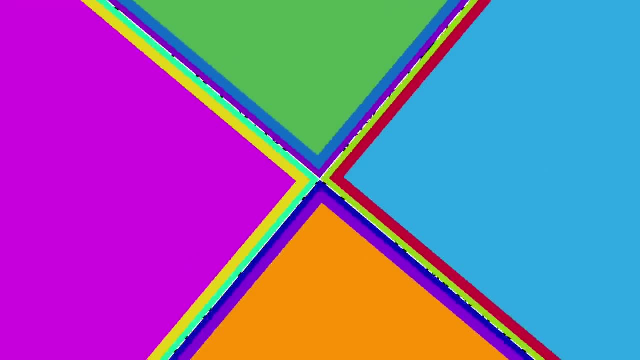 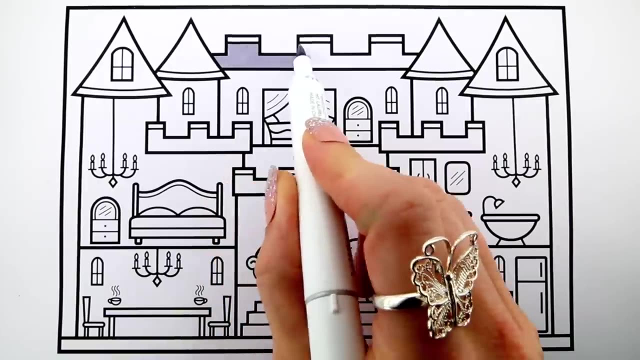 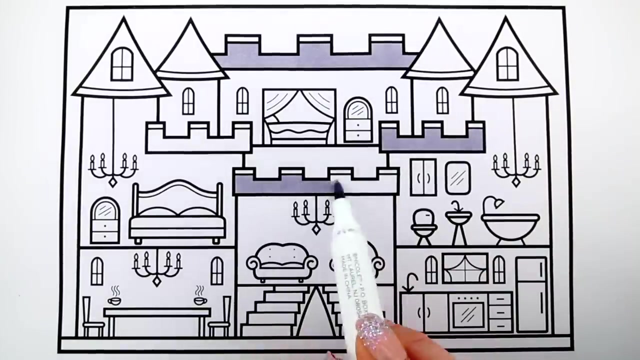 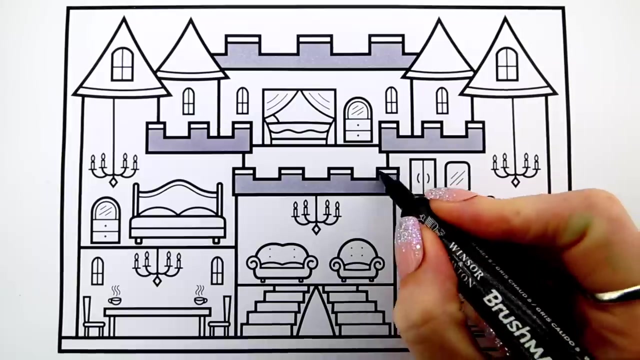 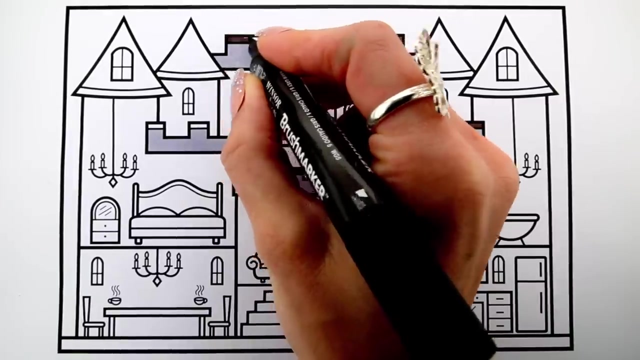 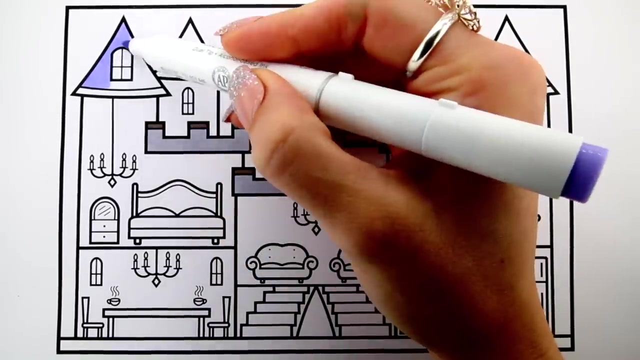 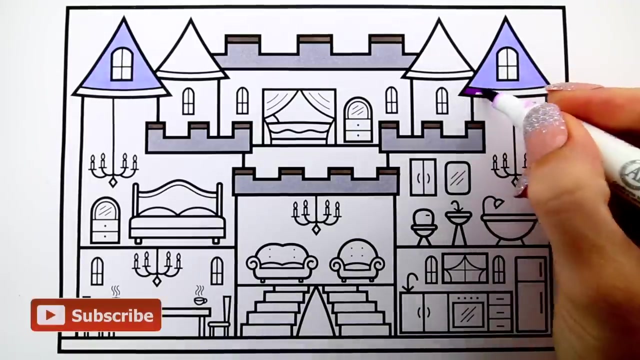 Hi everybody, Welcome to Colorful Creative Kids. Would you like to have some fun and color with us? If so, you're in the right place. Let's get started. If you're enjoying this video, please consider subscribing. and clicking the bell will let you know when we upload a new video. 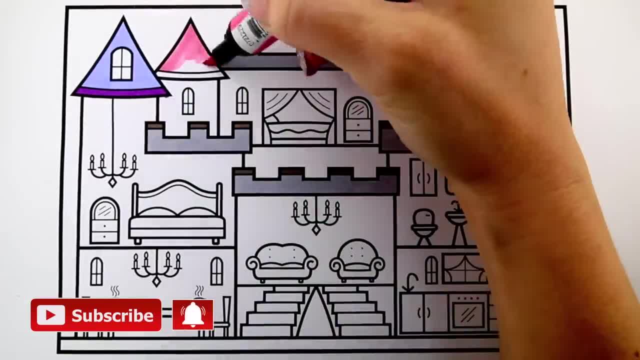 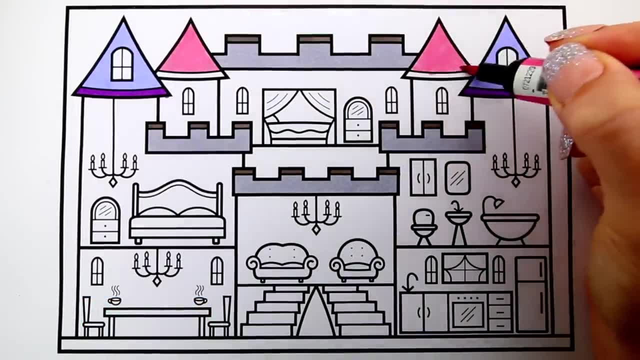 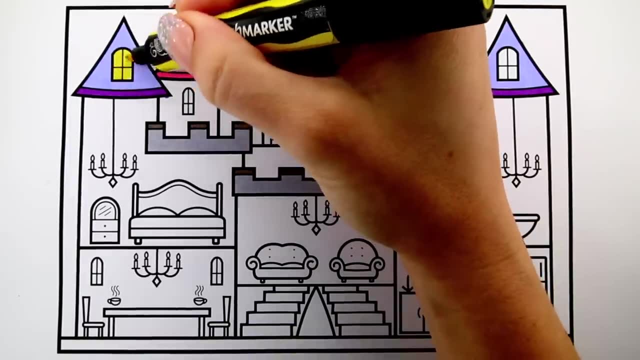 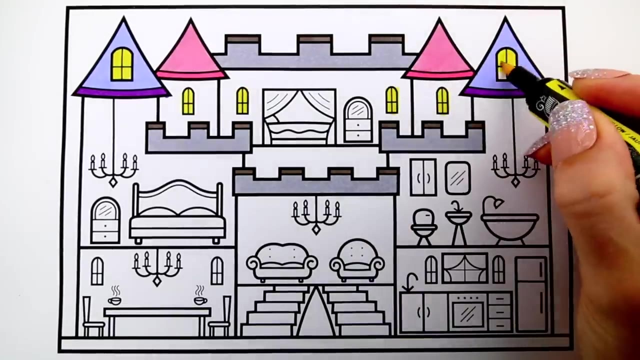 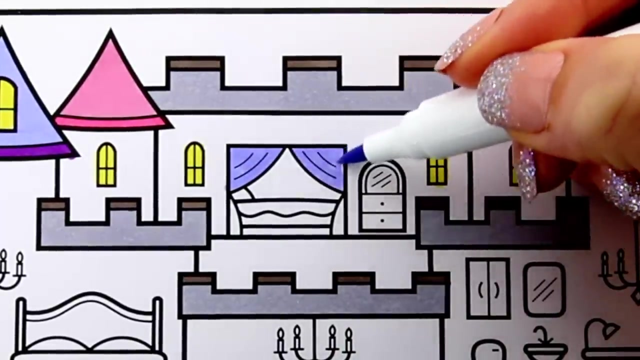 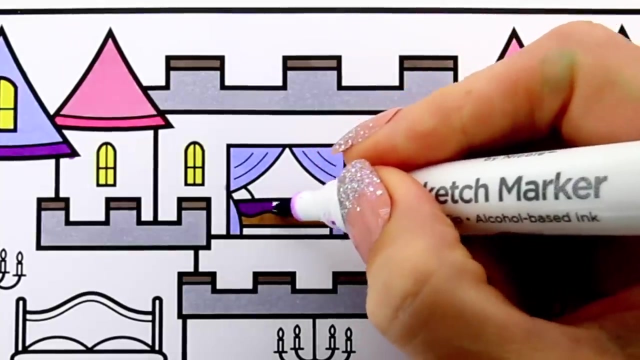 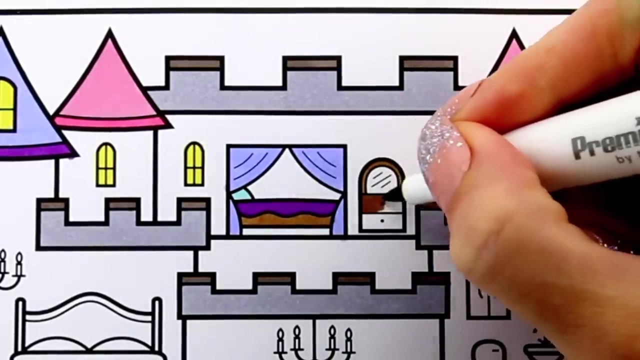 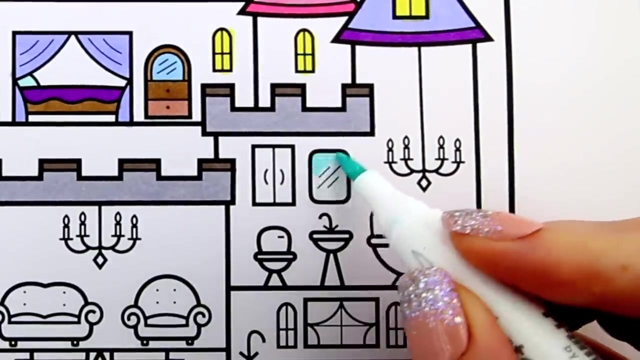 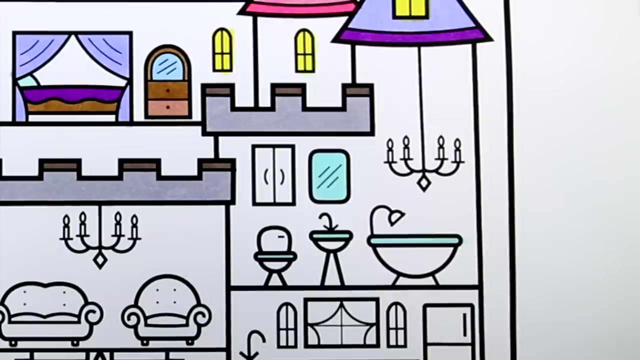 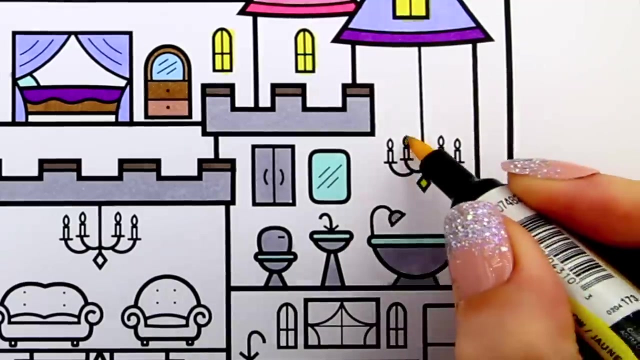 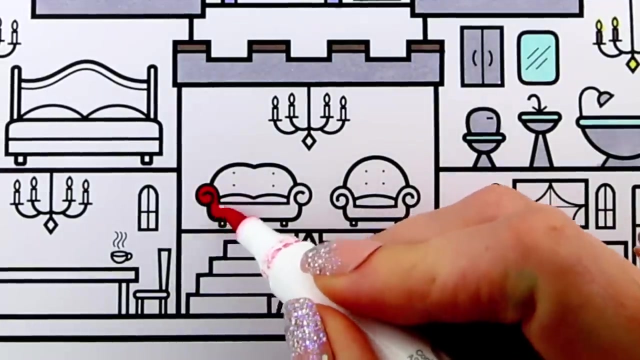 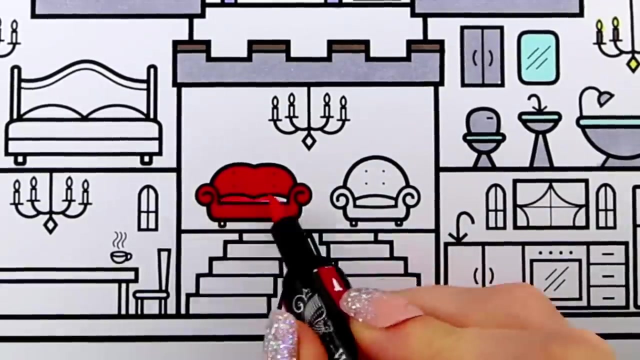 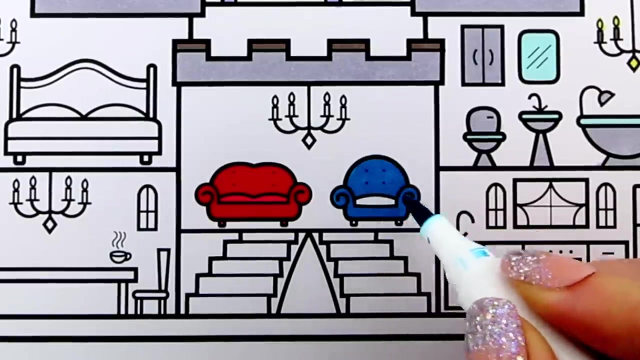 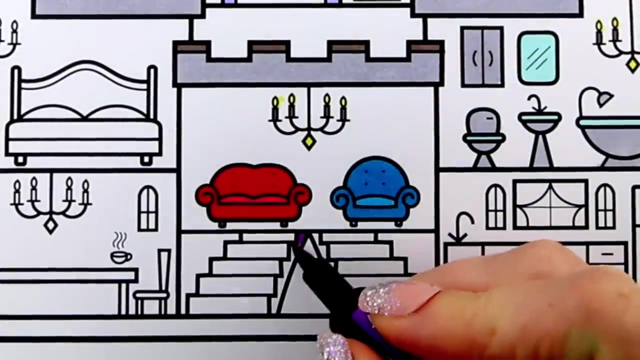 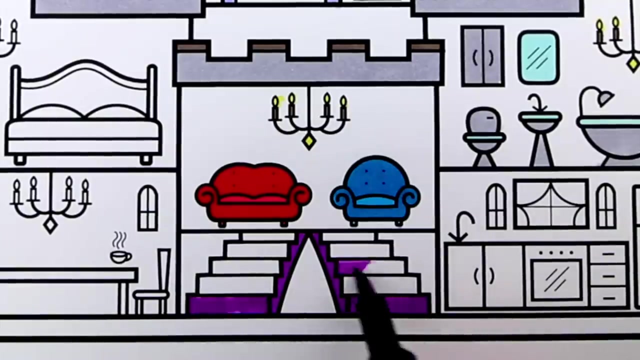 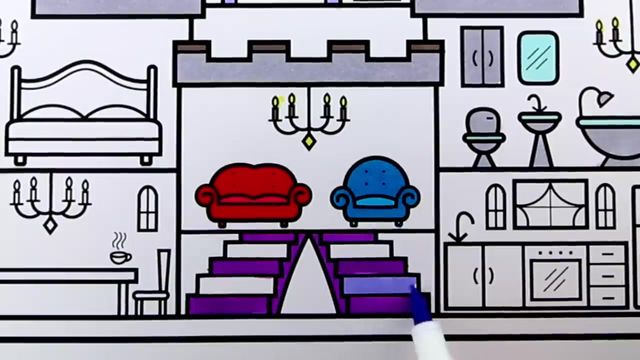 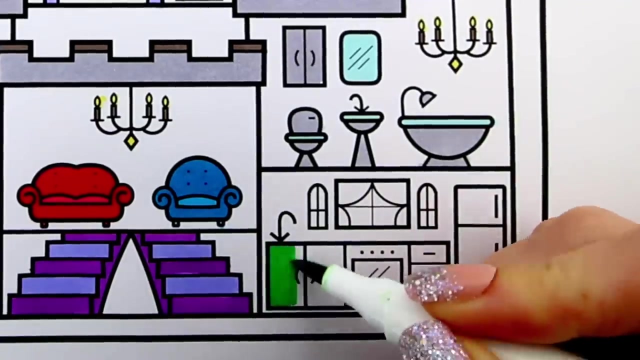 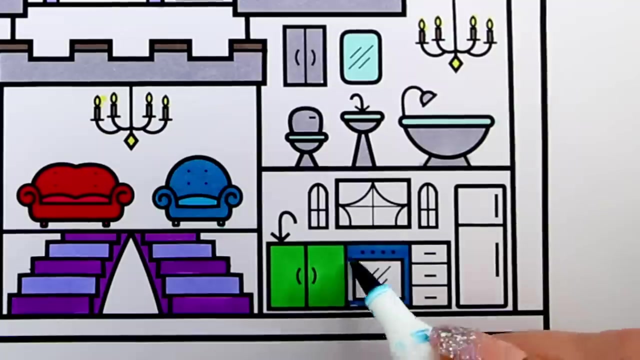 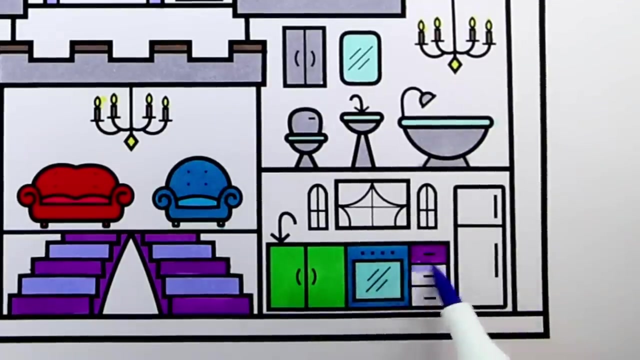 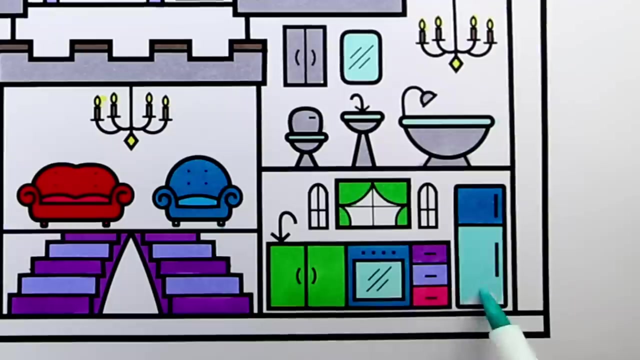 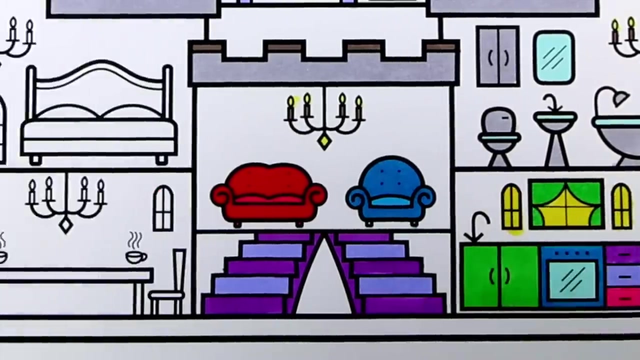 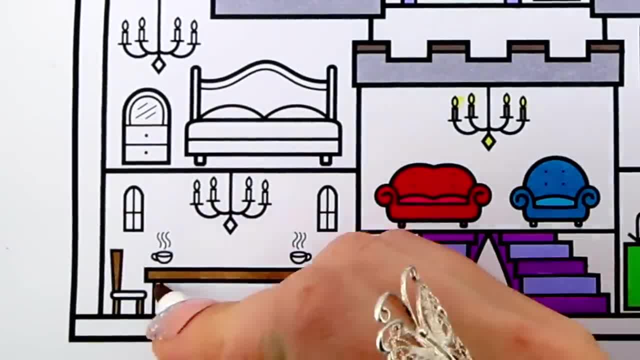 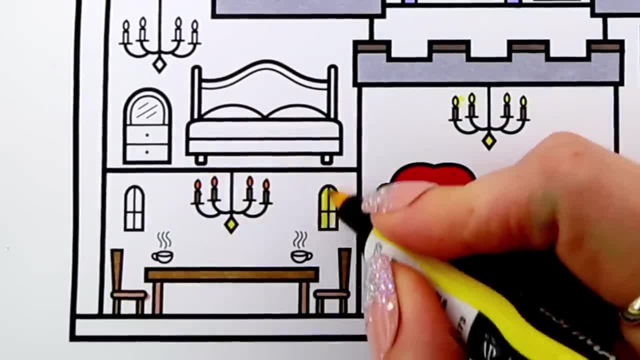 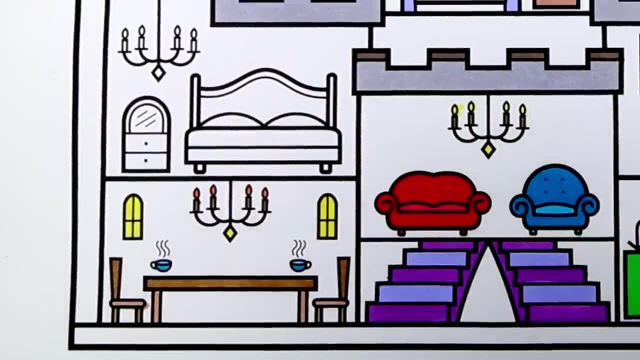 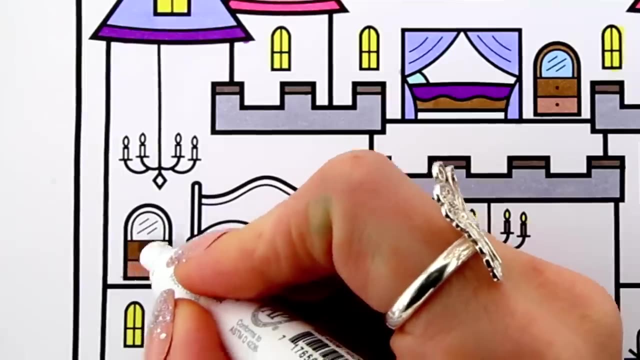 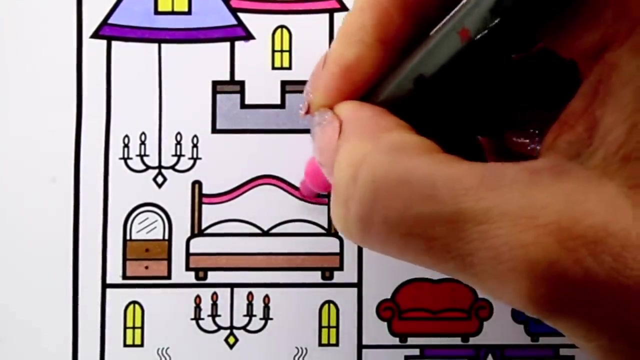 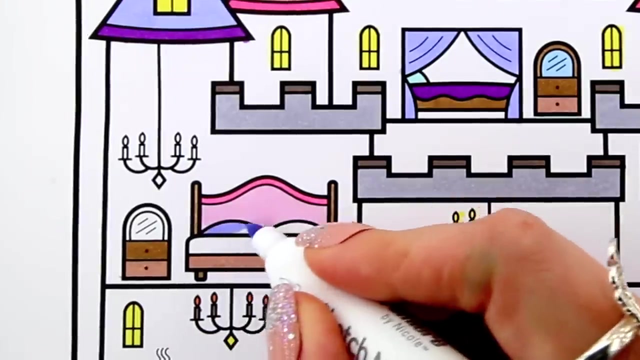 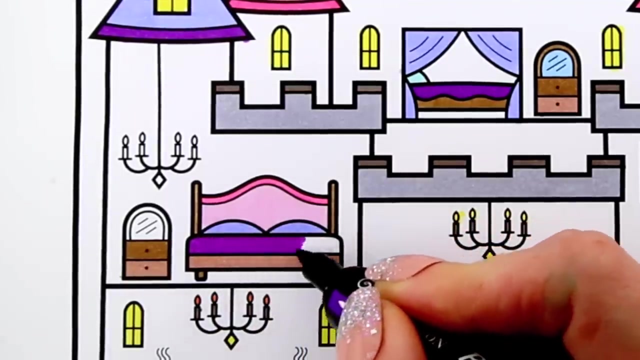 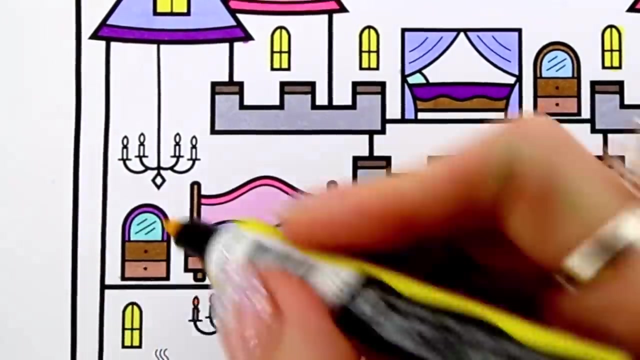 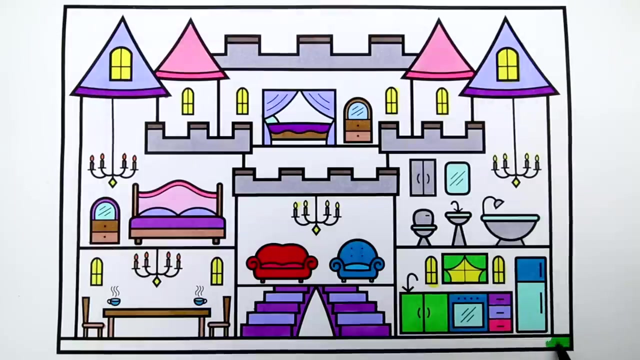 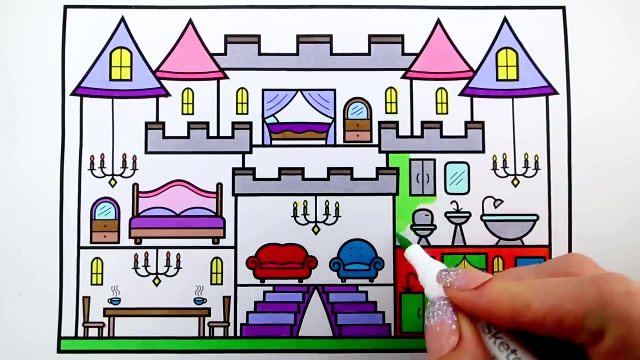 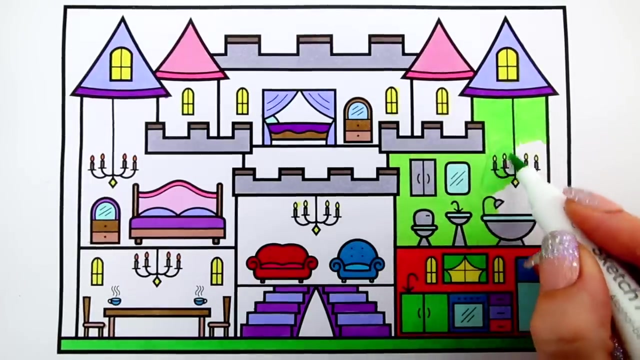 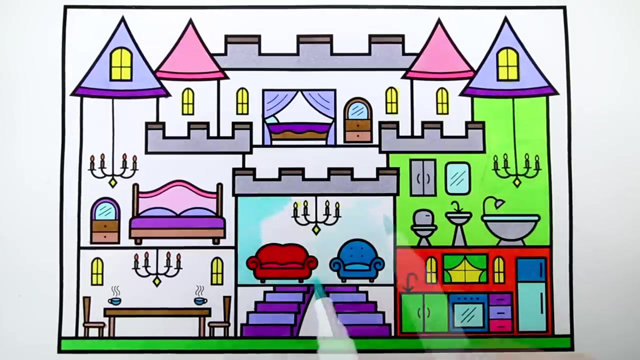 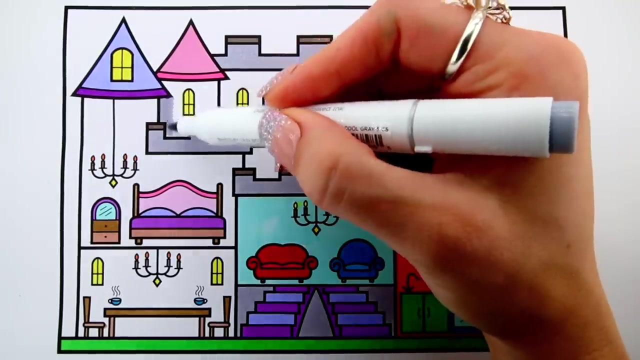 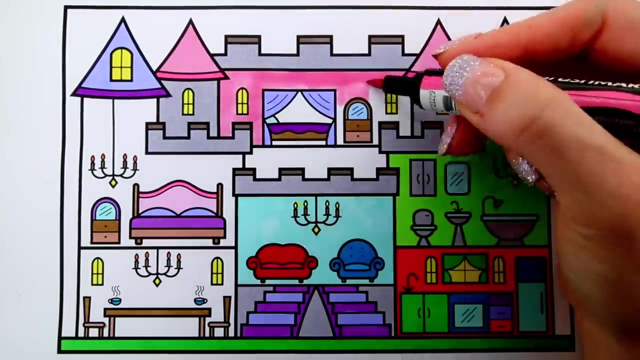 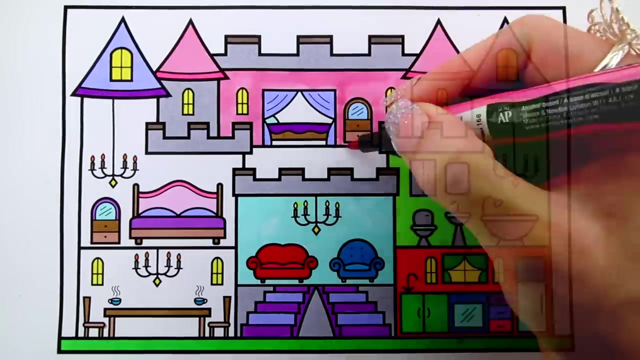 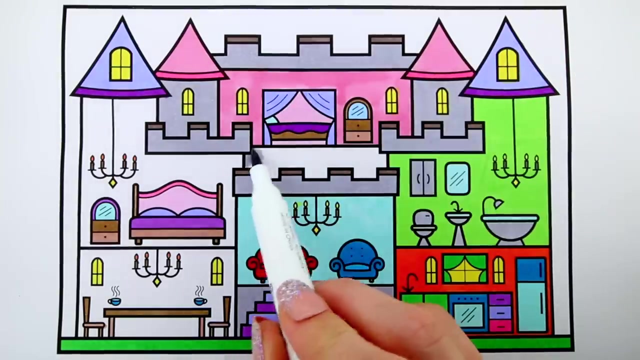 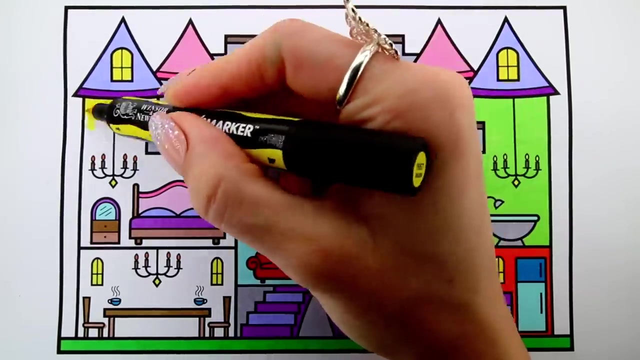 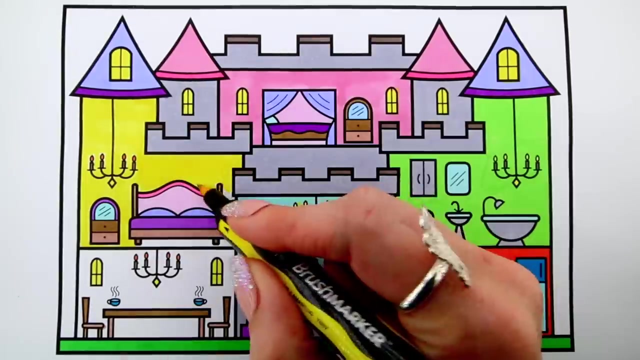 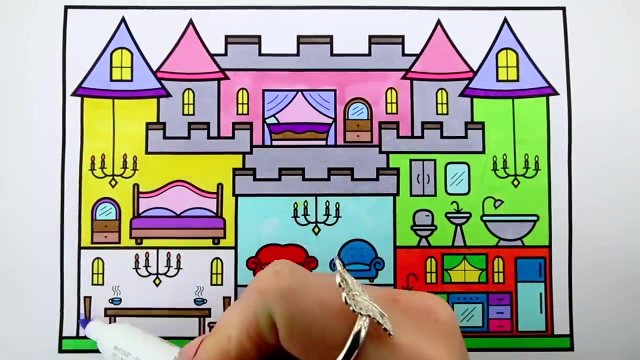 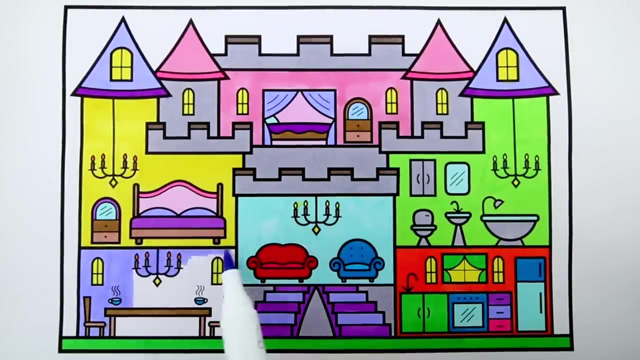 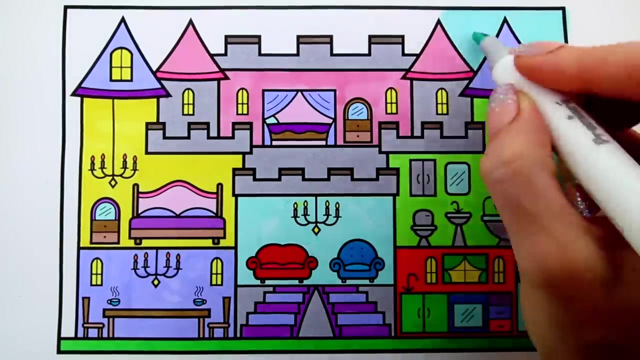 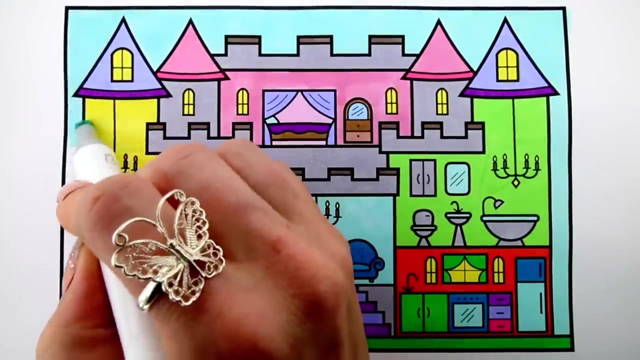 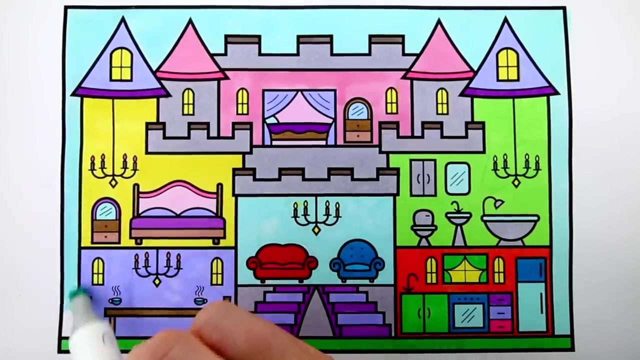 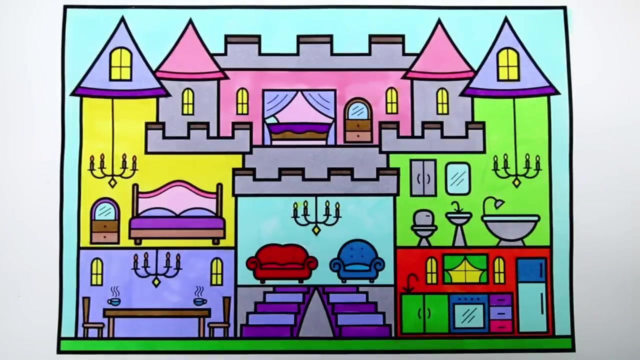 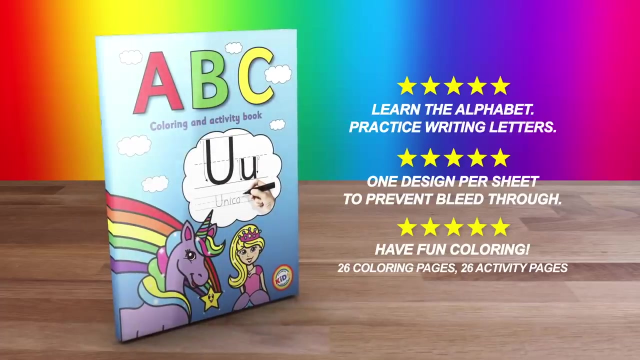